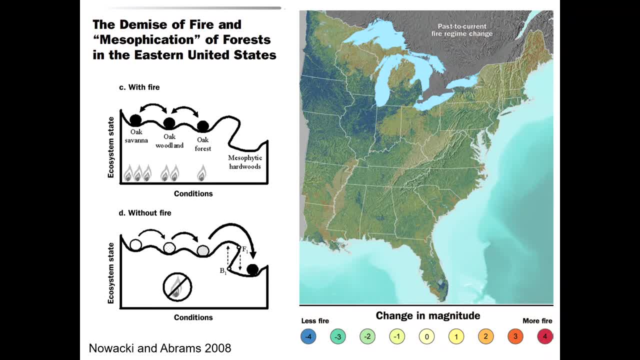 most areas in the eastern US have had reduced fire activity over time And this can lead to a problem essentially of forest being shifted from more of a xeric type of species composition to mesophytic species. So these are essentially called ball and cup diagrams showing the shift in these different ecosystem. 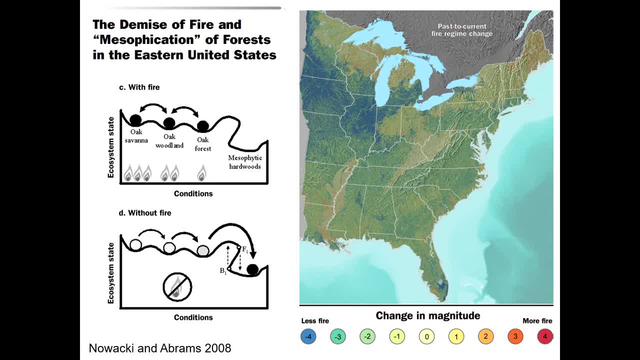 states and how hard it is to reverse a state from one to another position. So on the top here you can see that with different amounts of fire frequency, we tend to have oak, savannah, oak woodland, oak forest, And if we remove fire we drop into this area of mesophytic hardwoods And the distance 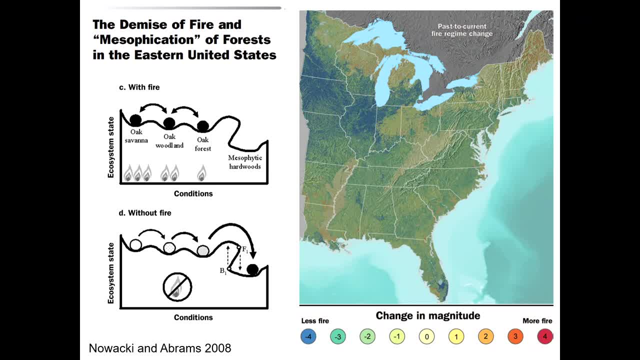 between this cup to this cup is the barrier to it. is this distance over this hump suggesting it's very hard to reverse this state? And that's shown further that when we remove fire from these systems, we drop systems into this mesophytic state and it's very hard to go back to an oak system, an oak-dominated 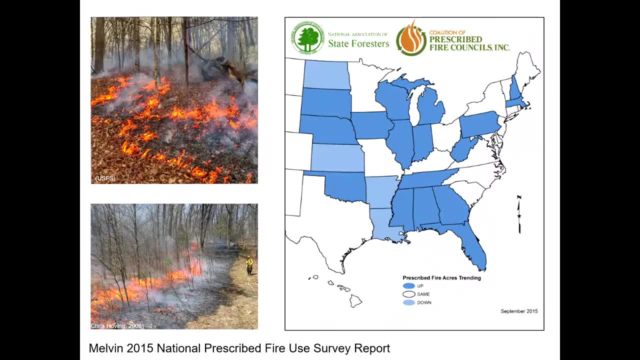 system. Okay. so fire clearly is important. We're recognizing this. We have lots of historical evidence to support it And that has all led to now an uptick in the amount of fire activity. So there's been a lot of interest in returning fire to the landscape. This is shown in this National Prescribed Fire Use Survey report. 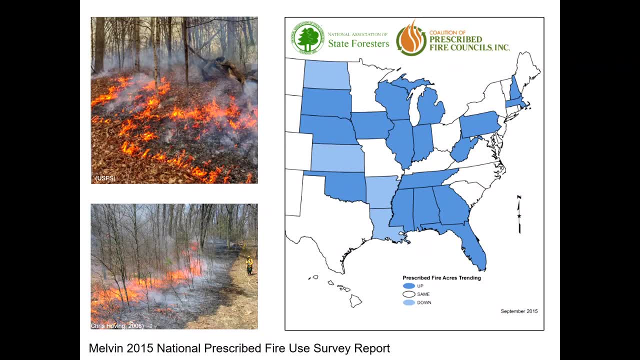 You can see again, Illinois has shown an increase in the amount of fire acres, so essentially places where there's surface fire activity, And I mentioned this is from 2015.. So over 3.6 million hectares of forest land in the US are currently. 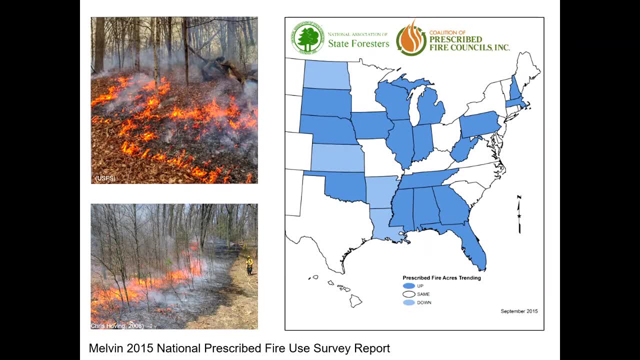 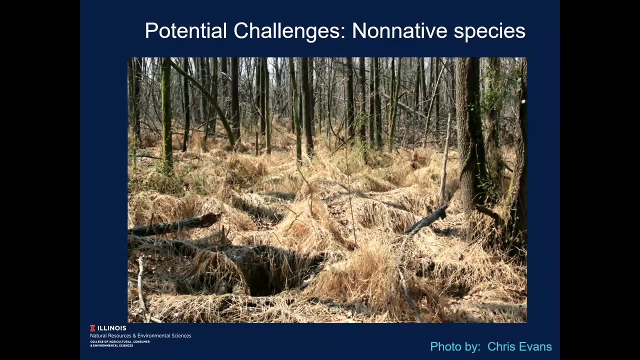 being burned, and a good portion of that is happening in Illinois. All right, this is an invasive species symposium. So here's where invasive species fit in right. They present a very significant challenge to returning fire to these landscapes. So one thing, and I'll. 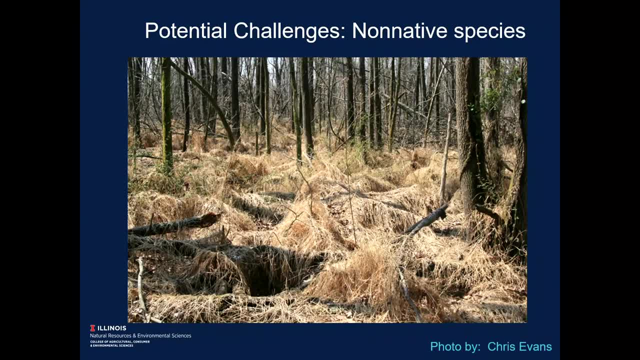 talk more in detail about this. now you can see it happens when we have invasives as we really change the potentially the fuel conditions in forests. So this is a photo from Chris Evans showing the invasion of Microstegium viminium, Japanese stiltgrass, which is a species I'll be talking about today. 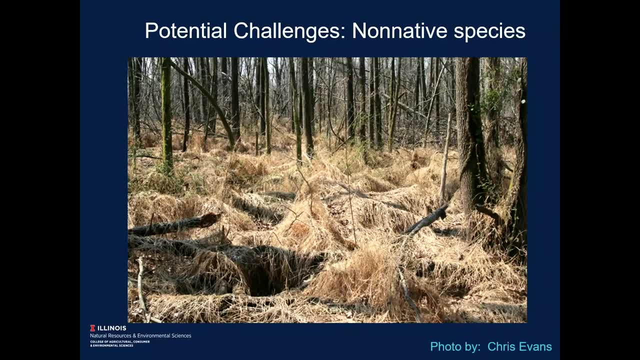 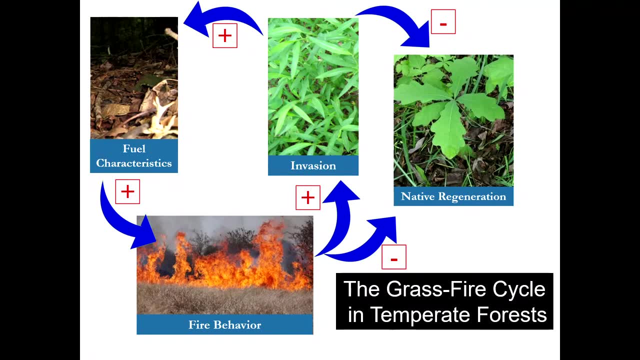 This is from Fort Massac in far southern Illinois. So the invasion of these systems, together with fire, can lead to what's referred to as the grass fire cycle. So let's just walk through this here. So a system that's invaded could be for a variety of reasons, but often it's been disturbed in some way. 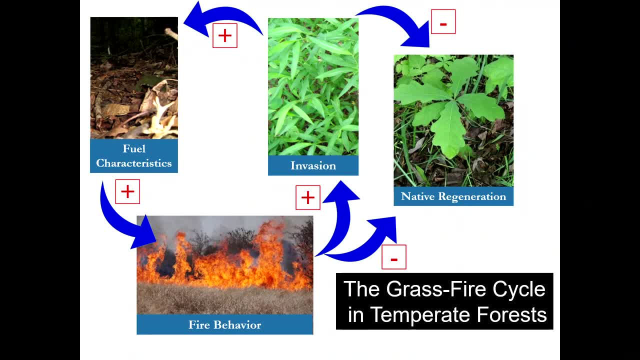 and that triggers the initial establishment of an invasive species, in this case, this annual grass microstegium that I'll talk more about in a minute And that can lead to an altered fuel load. It can increase the amount of fuels, but it also changes the architecture of those fuels. 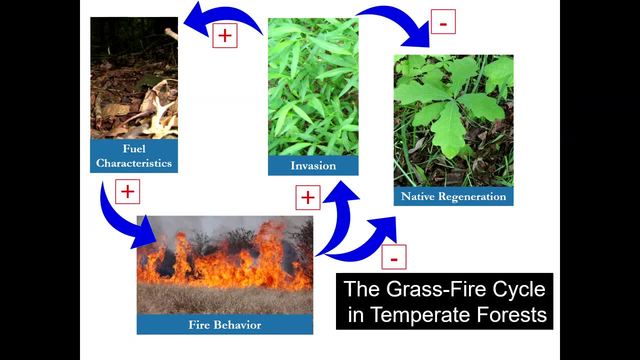 And that can lead to potentially higher fire intensity. so an overall change in fire behavior, a shift compared to what would have been the typical fire behavior without invasion, And that can have a couple different effects. One is it can actually lead to more severe invasions. 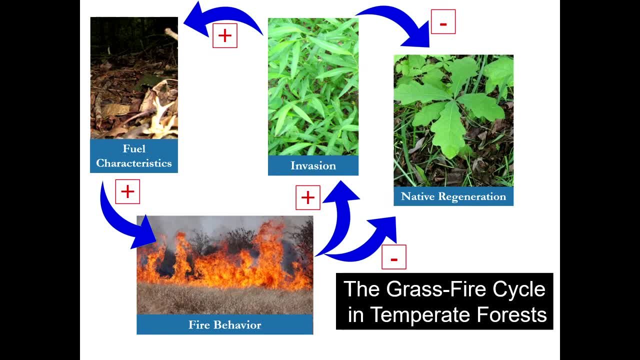 So I'll present evidence supporting that pathway- And it could also have this effect on the regeneration of native woody species. So that's particularly important in the sense that, again, if surface fires are being used to either maintain or restore these mixed oak systems, 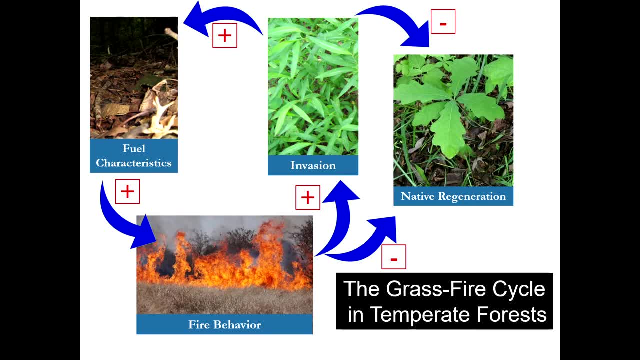 and now we have invasion leading to greater fire intensity that could have negative effects on the regeneration of native species. So it's a very important concern that led us to this body of research that I'll be discussing today. The other thing I want to mention is by promoting invasion, we could also have negative effects on native regeneration. 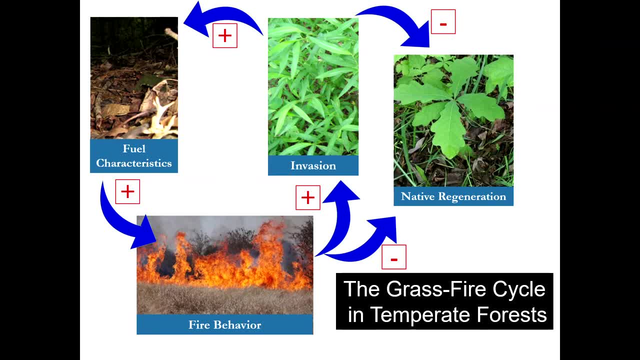 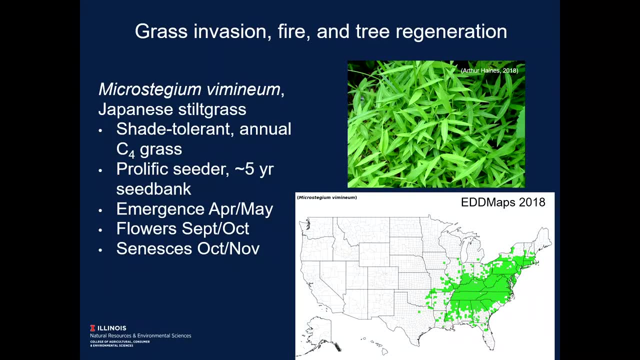 because there is this issue of competition that we've heard a little bit about already today, So I'll come back to that. Okay, so this is a species I'm going to talk about in the context of grass invasion, fire and tree regeneration. 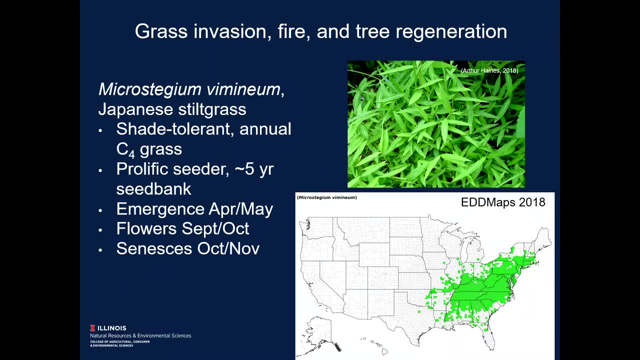 and that's Japanese stiltcress. So just to introduce you to the species if you don't know about it too much yet, it's a fairly shade-tolerant annual C4 grass. So most of our grasses in these systems are C3 grasses. 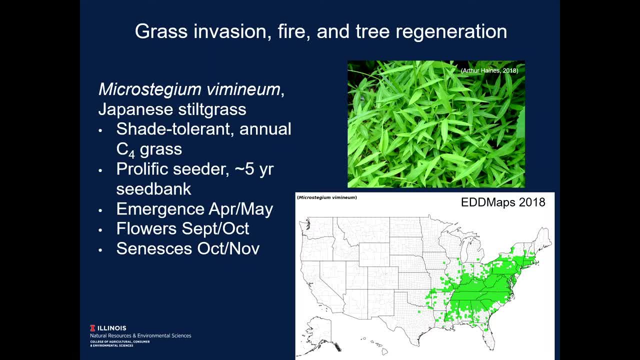 so this one's somewhat unique in terms of its photosynthetic pathway. It produces a lot of seed, which is probably part of the reason it's so successful, And the seeds persist in the seed bank for about five years. It also has some advantages in terms of its phenology. 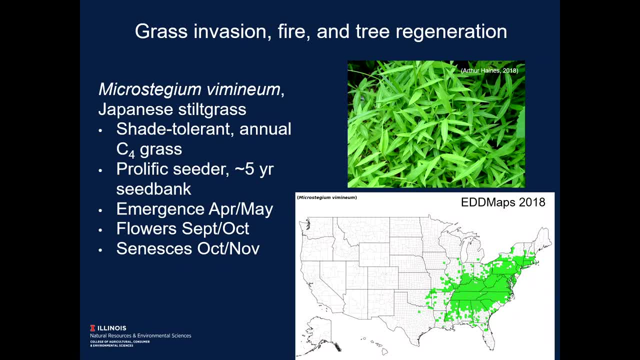 It greens up early, around April or May, so before a lot of other species are active in these systems, It can begin fixing carbon And then flowers late in the season- September, October- and doesn't senesce until October, November. 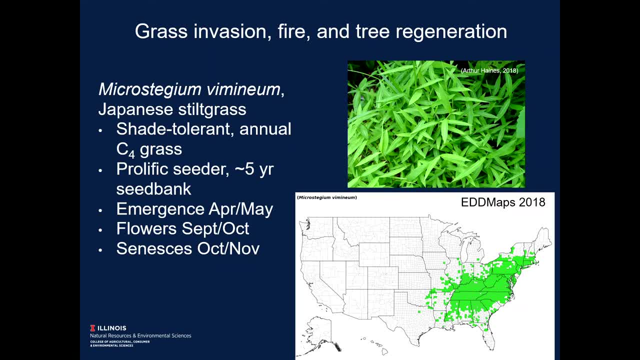 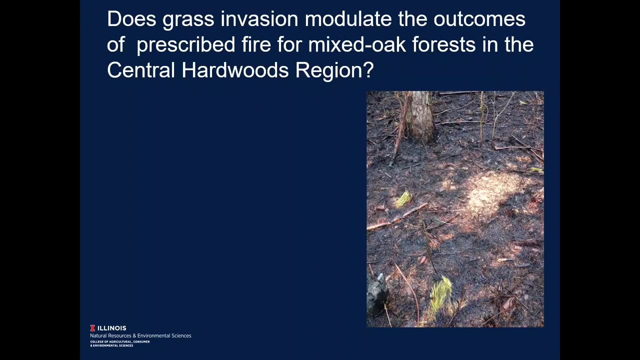 So it has this extended period of time over which it's biologically active, And I should mention that it's native to Asia and was introduced to the US in 1920 as packing material. So again, I'm going to present results from a couple of different studies. 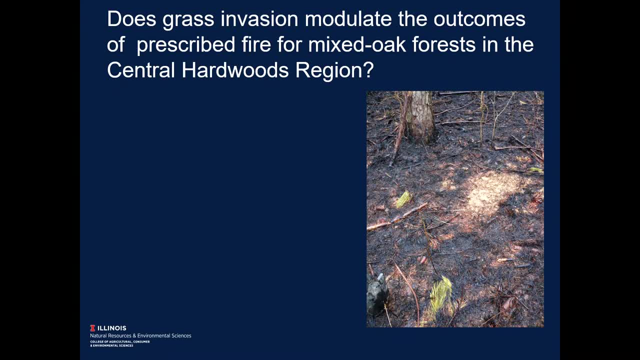 The overall question here being addressed is: does grass invasion modulate the outcomes of prescribed fire for mixed oak forests in the central hardwoods region? So the first question I'll be presenting results with is: how does grass invasion affect fuels, fire behavior, grass performance? 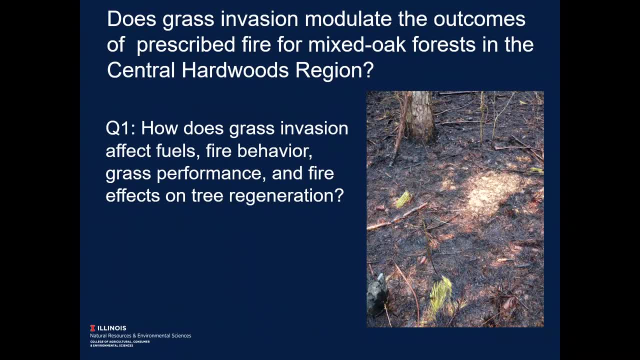 and then the fire effects on tree regeneration, And then I'll also talk about if we repeatedly burn areas. does that have different outcomes in terms of this feedback between invasion and fire, Since repeated fire is one of the main management strategies being used by land managers? 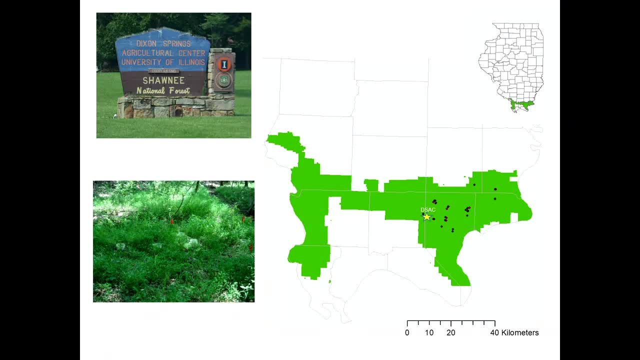 So this work I'm going to talk about was all conducted in southern Illinois. The first set of studies were conducted mainly in the eastern portion of the Shawnee National Forest at a range of different sites, but primarily in Pope County, Illinois, And then in subsequent studies we've worked in other parts of the other counties to the west. 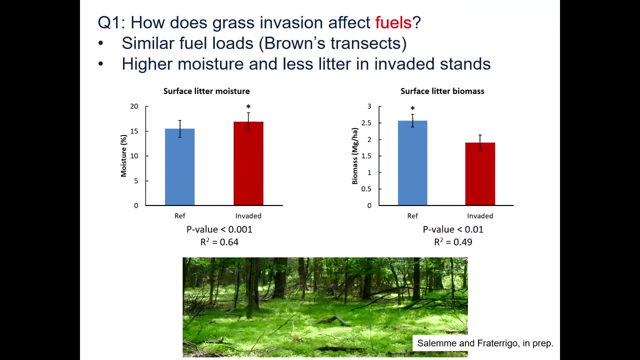 So I'll talk about that in a minute. Okay, I'm going to just jump right in then with some results. So the first part of this is again: how do fuels change? And there are many different ways to measure fuels. We quantified fuel loads. 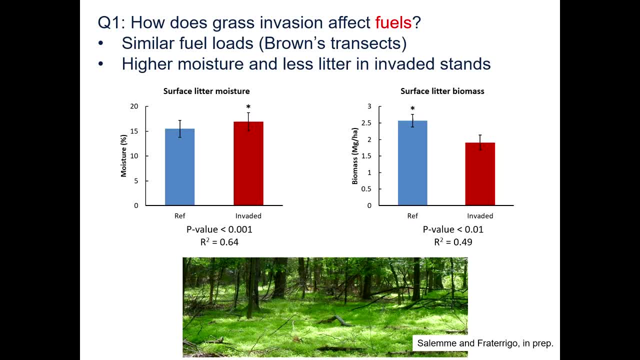 This is woody fuels in particular. using Brown's transects, We basically saw no difference in terms of the amount of woody fuels or the composition of woody fuels in these invaded and uninvaded areas. So the blue would be the uninvaded reference areas. 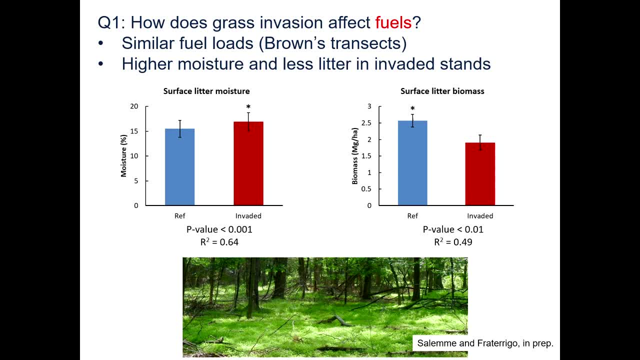 and the red bars here would be our invaded areas. But we did see differences in terms of the environmental conditions and the litter moisture that correspond with the types of conditions or habitats in which stiltgrass is most successful. So we saw essentially stiltgrass being 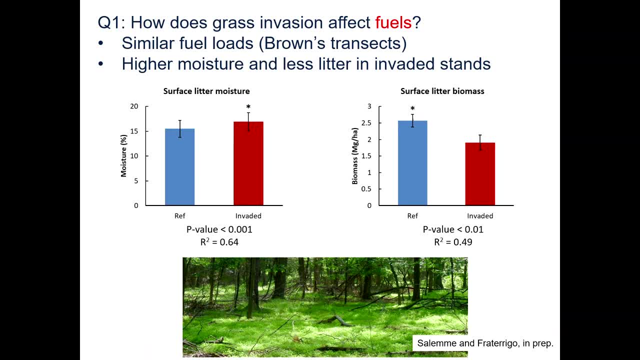 invaded areas having higher litter moisture, and we know that already. stiltgrass does well in these high moisture conditions, so that didn't really come as a surprise. We also found that stiltgrass was more abundant in places where litter biomass was lower. 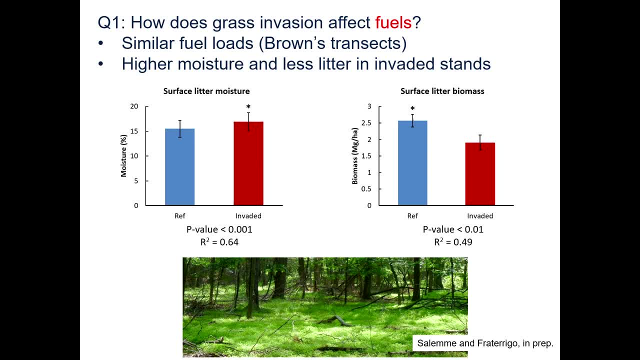 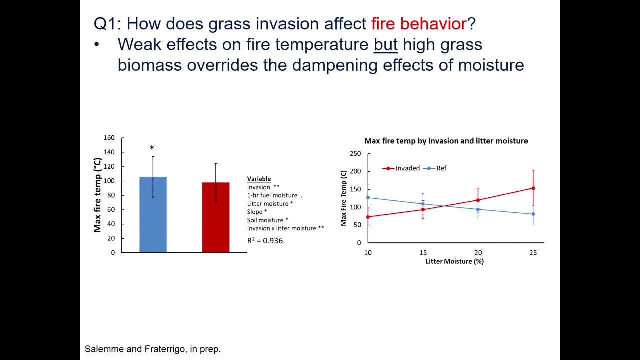 Again, not a surprise. Previous studies have shown that where the forest floor is lower, thinner, then we see higher levels of invasion. Okay, so what does this mean for fire behavior? So if we try to link information about the fuels, we didn't see any strong differences in fuels. 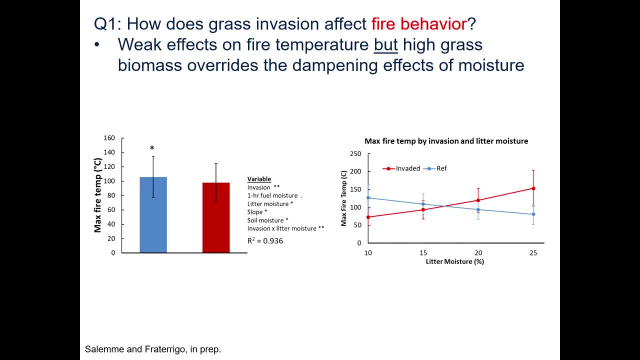 but again, those Brown's transects focus on woody fuels, but we know that the senescent material of microstudium itself can affect fire. What do we see? Well, when we just look at maximum fire temperature in degrees Celsius, 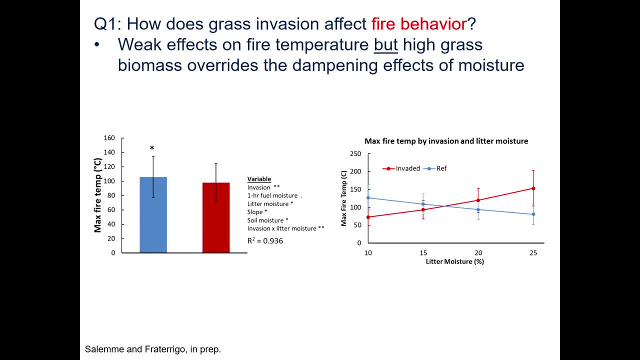 we actually see higher maximum fire temperatures in our uninvaded stands. I will mention that when this study was conducted it wasn't a great year for fire. It was less conducive, It had been wet and kind of cool when the fires were being conducted. 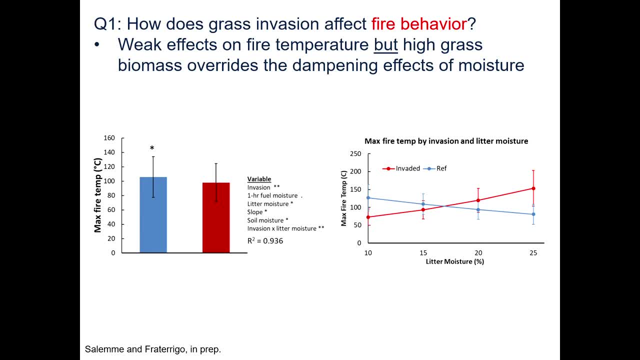 and this, I should mention too, was done together with the burn crew in the Shawnee National Forest, so we were just kind of choosing sites that they had already, you know, the sites that they had already planned to burn, and so this would have been their typical burn regime in these forests. 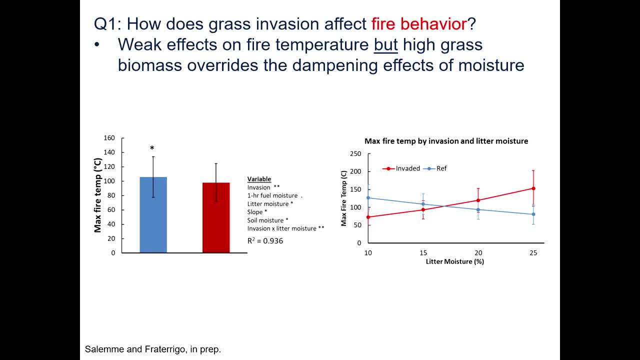 So overall we see lower maximum fire temperatures in invaded stands and if we look at these data continuously we see, as we would expect again in the reference stands, overall, as moisture increases, fire temperature declines. That certainly makes sense. 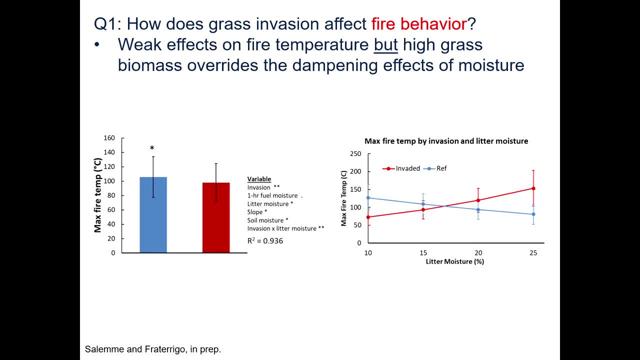 The opposite pattern, though, was true for invaded areas, And what we think is happening again in these high-moisture areas, that's where we actually see greater biomass. So we think that you know eventually, as we get to high-moisture, high-biomass conditions, 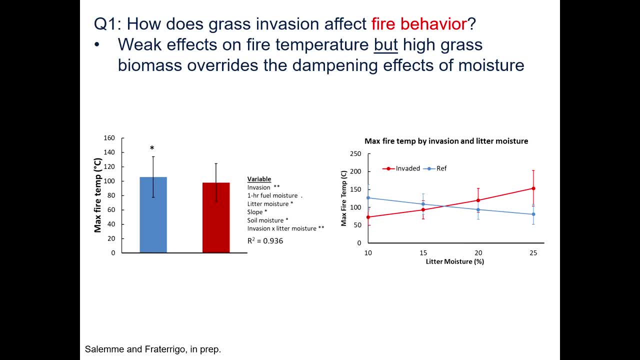 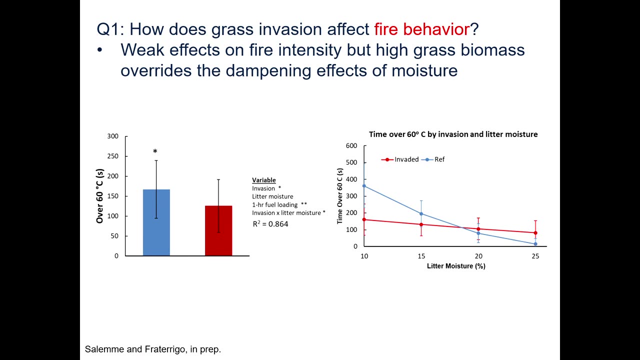 that overrides that dampening effect of moisture on fire. So it is possible, or we do see evidence, to suggest that higher microstudium biomass can lead to greater fire intensity. We see sort of weaker patterns when we look at residence time. So this would be the amount of time. 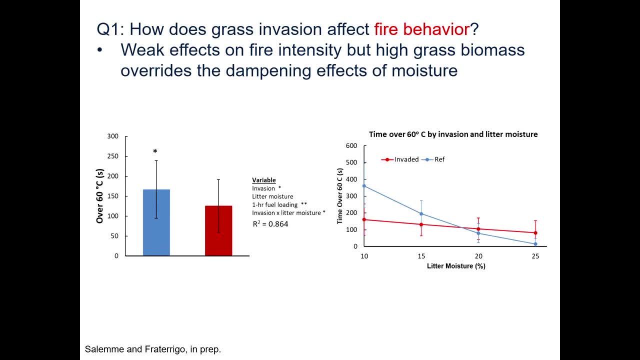 that a fire burns really hot, In this case over 60 degrees Celsius, which is the temperature at which plant cell death can occur. So this is an important threshold And again, we see higher residence times for the uninvaded stands as compared to the invaded stands. 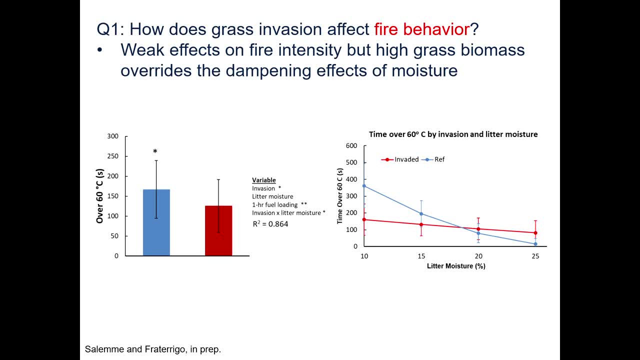 but a very similar pattern in that that declines in the reference stands with high moisture or with increasing moisture and it's a lot shallower, steeper gradient for the invaded stands. So we see higher residence times for the uninvaded areas and getting to the point where we have high biomass. 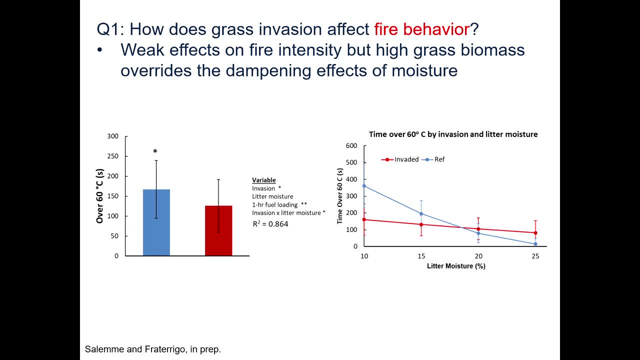 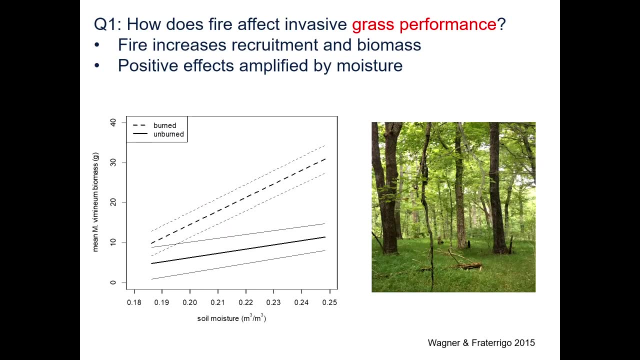 under these high litter-moisture conditions. we see actually the residence time creep up a little bit over the reference conditions. Okay, what does this mean in terms of how it affects future invasion Again? so this idea of the feedback between fire and invasion, 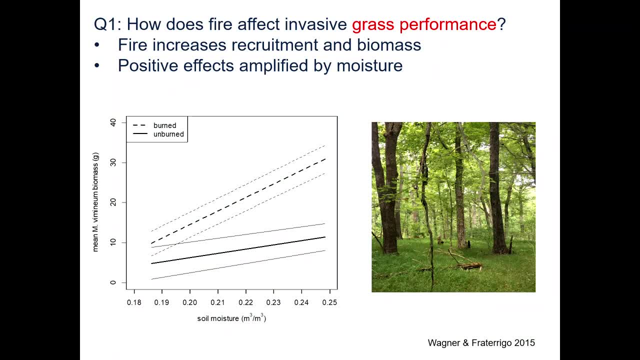 This is work from a previous graduate student, Stephanie Wagner, and we found that overall, fire does, in fact, promote invasion. We see higher- this is biomass of microstegium-vaminium. We see higher biomass in burned areas shown by the dashed line here. 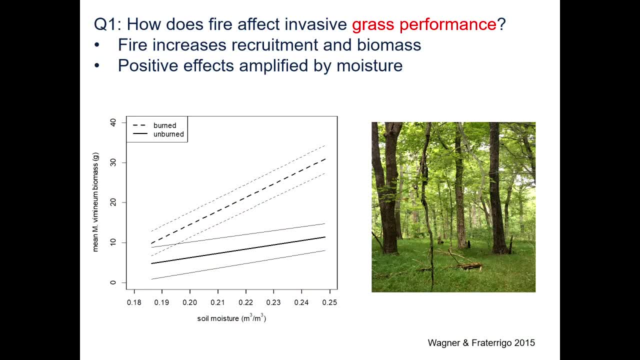 and you can see that's amplified with soil moisture, which is on the x-axis here. So higher soil moisture in these sites that are burned leads to very, very big flushes of biomass following the fire in the next growing season. Okay, so this is sort of this effect of fire. 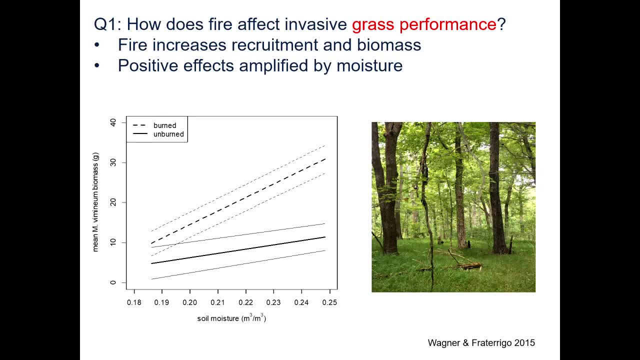 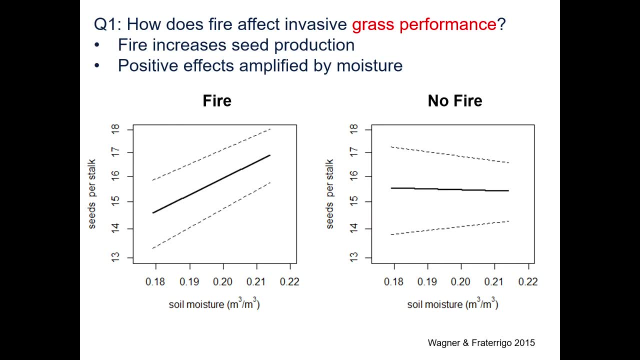 from one growing season to the next, and you can see it's a much flatter slope for our unburned stands. We also measure performance in terms of seed production, So again telling us something about whether or not this invasion will be maintained, since this is an annual plant. 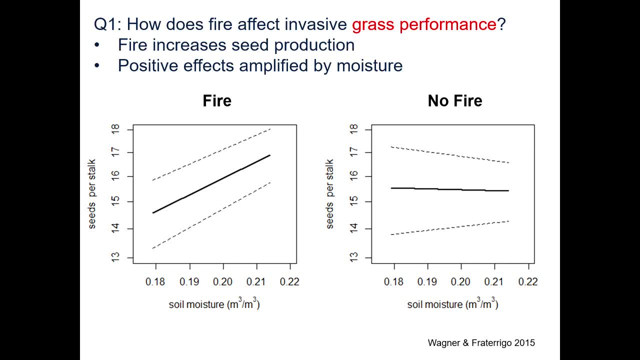 Seed production is critical And again seeds per stock increased pretty steeply in the burned areas with soil moisture and we see a much flatter type of response with soil moisture under those conditions where there was no burning. So again, overall, suggesting fire is having positive effects. 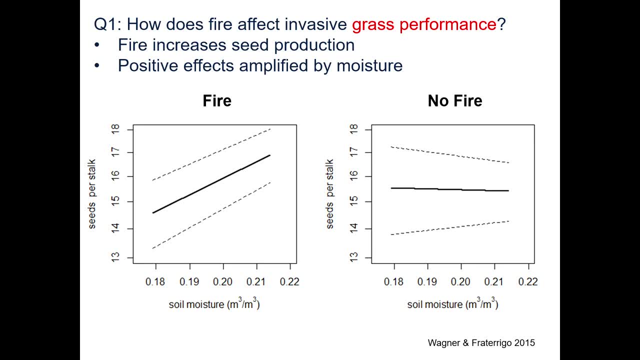 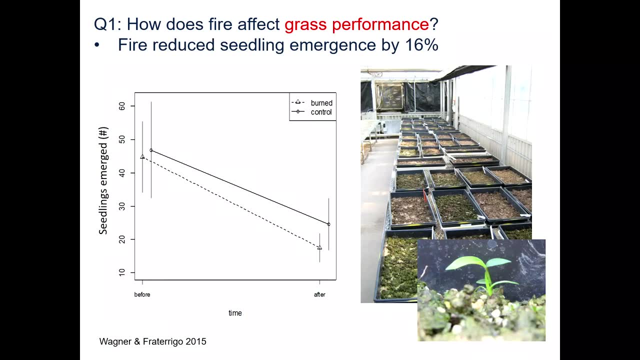 on the biomass and the seed production, the overall performance of Japanese stiltgrass, which is amplified by moisture. If we look at whether fire reduces the seed bank in any way, which we may think is a positive thing, right, we unfortunately don't see much support for that. 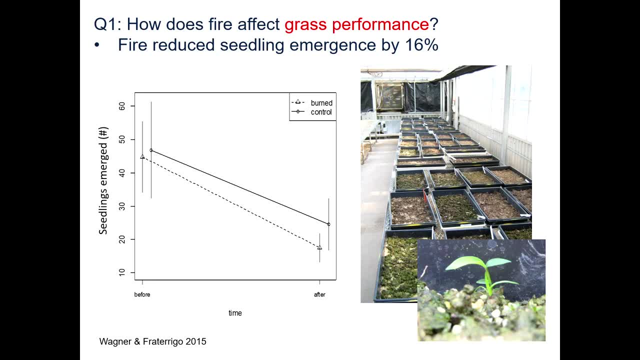 So we did some germination trials in the greenhouse, where we collected soils from areas that had been invaded and either burned or didn't burn, and the top solid line is the control and the bottom dashed line is the stands that burned. So, from before the fire till after the fire, 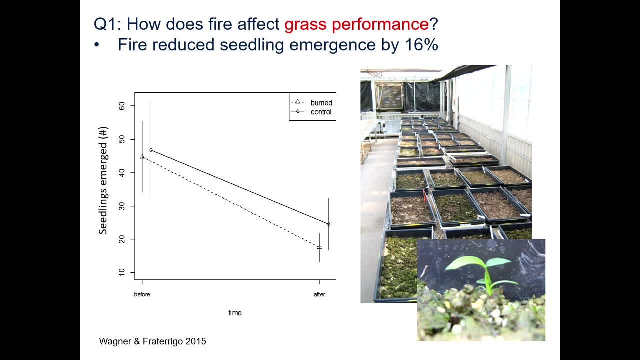 we did see a decline in seedling emergence, but that was pretty much matched by the overall effect of time of seedling emergence in the non-burned stands. suggesting fire isn't really having much of an effect on the seed bank at all. 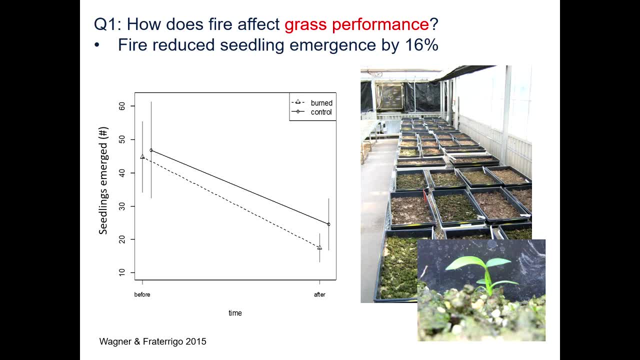 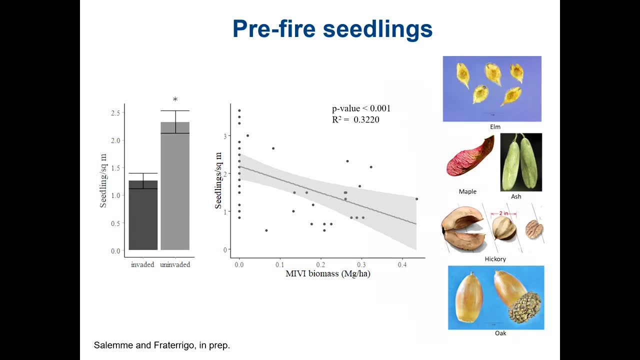 And these again are low intensity surface fires, so it's quite possible they're just not getting hot enough to kill these seeds and make them non-viable. Okay, so now I want to talk about the woody natives, since that was one of the things I mentioned. 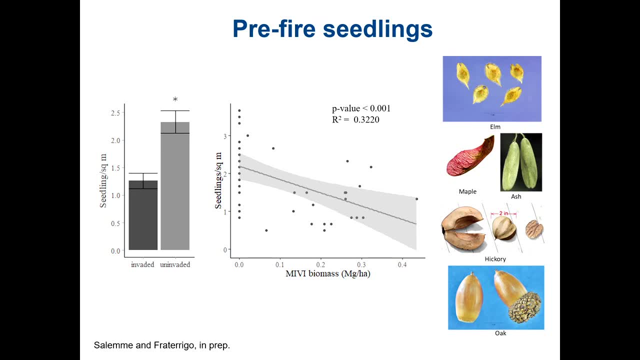 as an important reason for this study. So if we just look at before fire, what's the relationship between invasion and the amount or density of seedlings- woody seedlings. So this is across all the species that we encountered. This is seedlings per square meter. 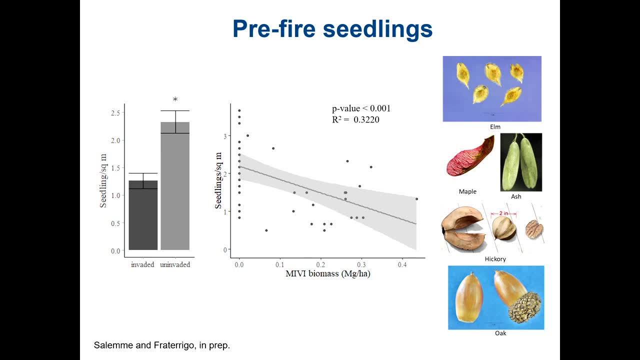 and you can see there's an overall negative relationship between stiltgrass biomass and the number of seedlings in a given area, suggesting again there's some negative effect of the invasive species abundance- Japanese stiltgrass abundance- on woody seedlings. 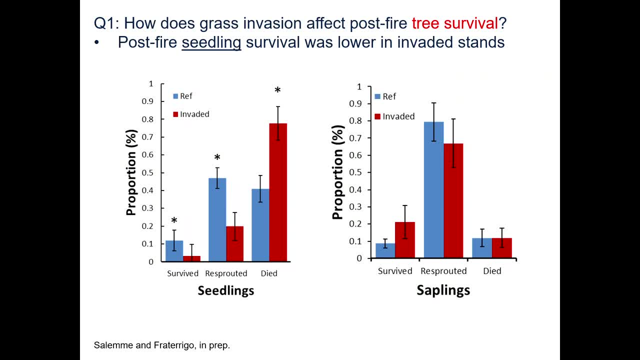 What if we look at this between fire events? So we tagged individuals and then tagged them before fire and then went back and remeasured them, so located them again and remeasured to determine whether they had persisted either in terms of overall survival, evidence for resprouting. 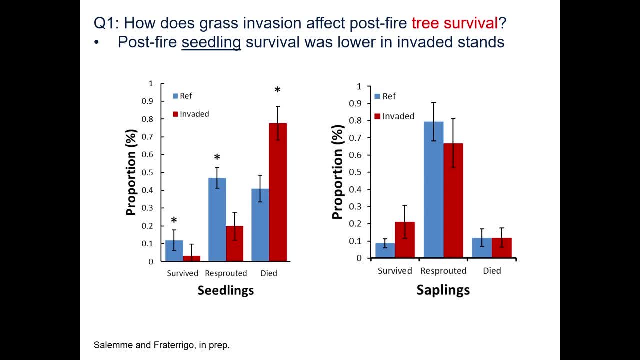 or whether they died, And we see that in the invaded areas survival level of resprouting was lower. So this is post-fire, suggesting that invasion and fire together leads to an overall decline in the number of or the proportion of native woody species. 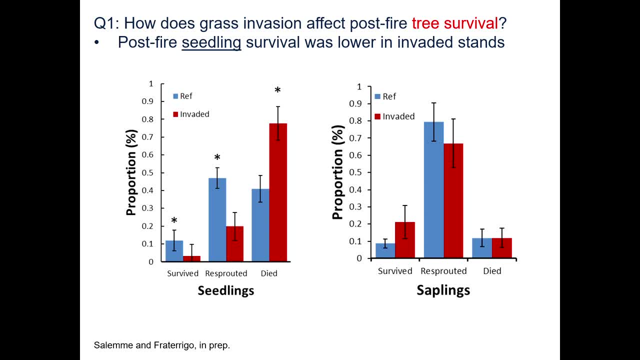 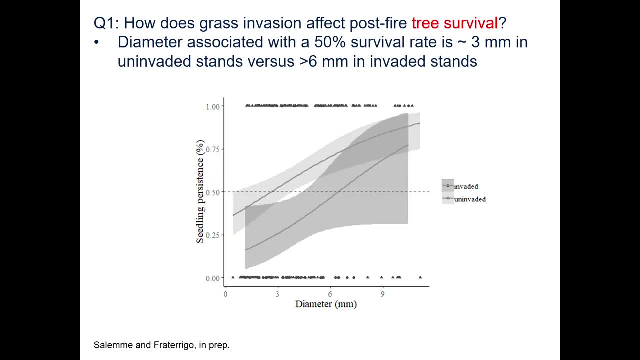 And you can also see the increase in the number that died due to that fire. So there is some positive news, I guess, on this front, and that is that the size of those individuals really had a strong effect on whether or not it was able to survive the fire. 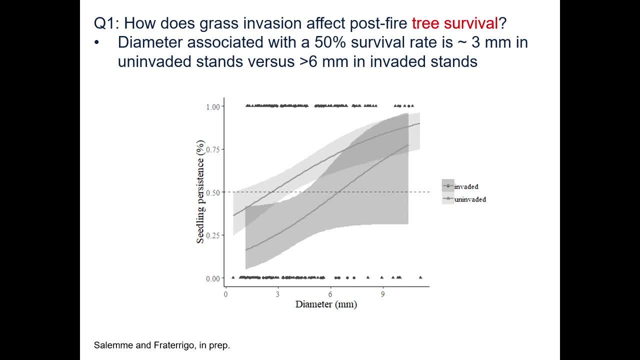 So overall we saw that larger individuals were able to tolerate or withstand fire even in the invaded stands. So this is diameter on the x-axis and persistence again from that pre-fire to post-fire time. And I just added the one thing I wanted to draw your attention to. 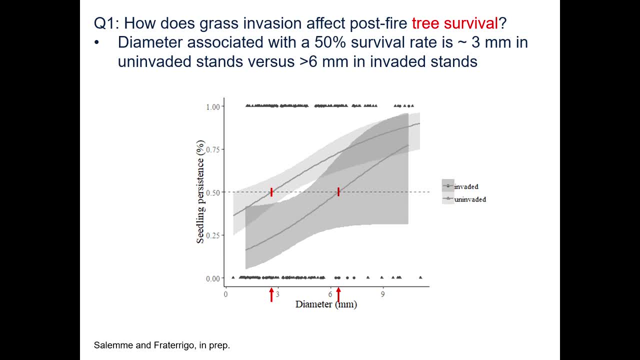 was essentially- that you know- 50%, so about half of the individual's survival rate. here you can see is around 3 meters and diameter size seedlings for the unburned condition. I'm sorry for the uninvaded conditions. 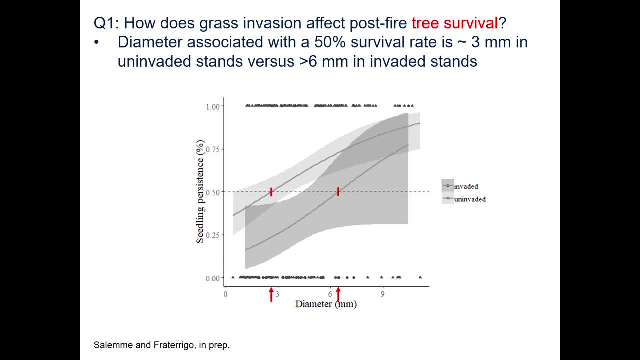 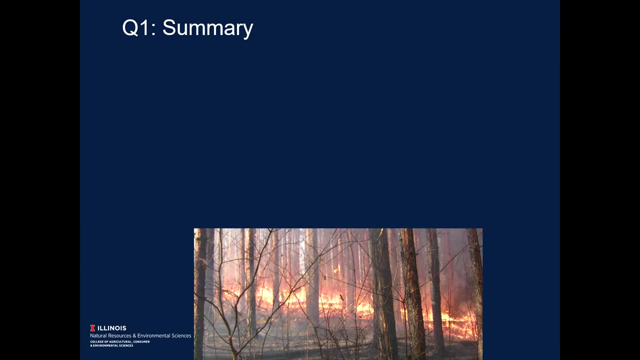 and for the invaded conditions, you have to be quite a bit larger to reach that 50% survival rate. Okay, so there is a doubling approximately of the size that's required to survive, or suggest survival, at 50% levels. Okay, so just to summarize: 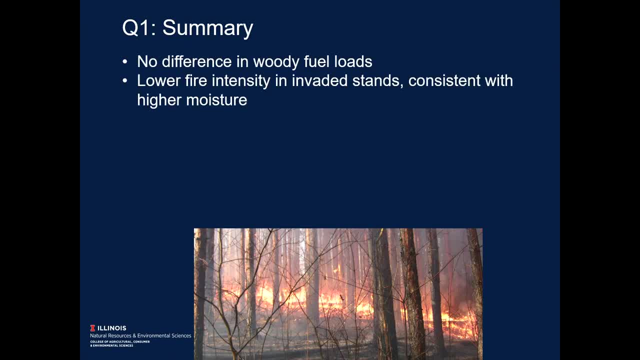 no difference in those woody fuel loads and overall lower fire intensity in the invaded stands consistent with the higher moisture conditions and higher microstegium invasion. positive feedback between fire and grass invasions, again moisture amplifying this effect. 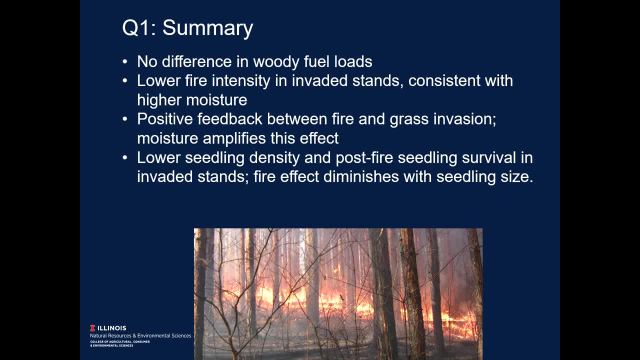 And lower seedling density and post-fire seedling survival in the invaded stands. So the fire effect diminishes, though with seedling size. So you might be scratching your head, though, at these two results, because they seem a little bit counterintuitive. 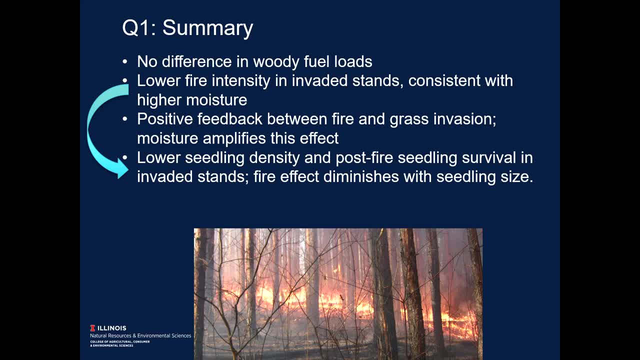 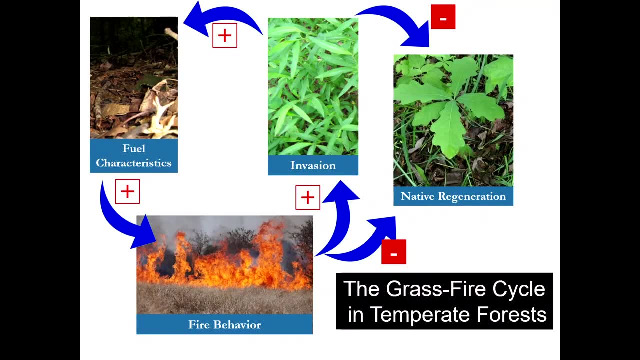 Lower fire intensity in invaded stands and yet lower post-fire survival. Why is that So? one of the things I mentioned early on is that we can imagine that this increase in fire intensity can have negative effects on survival. right, That's one pathway by which invasion and fire interact. 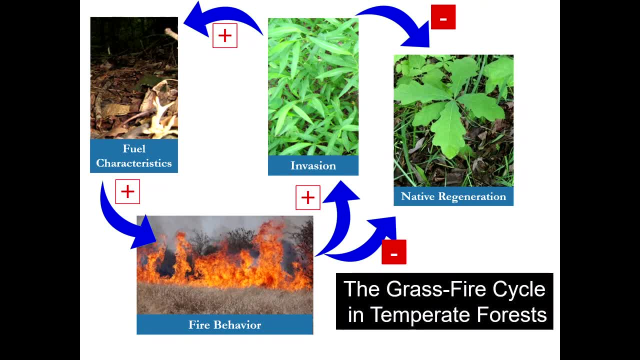 to affect native regeneration. But another pathway again that I mentioned is these direct effects of invasion. So if fire promotes invasion, this could also have very negative effects just through, say, resource competition. So we wanted to try to use our data. 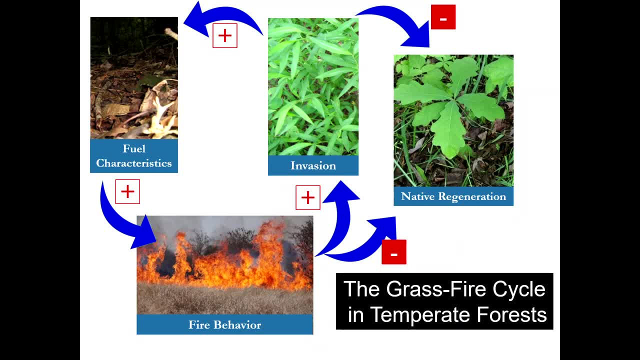 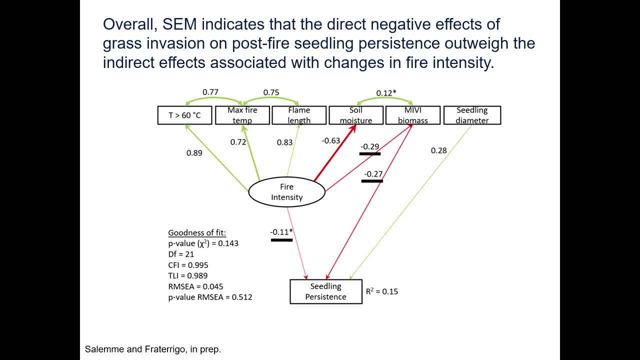 to address whether one of those two pathways was more supported, And we found evidence, or support for this idea, that those direct effects are actually playing a bigger role in persistence than fire intensity. So this is a structural equation model. There's a lot going on here. 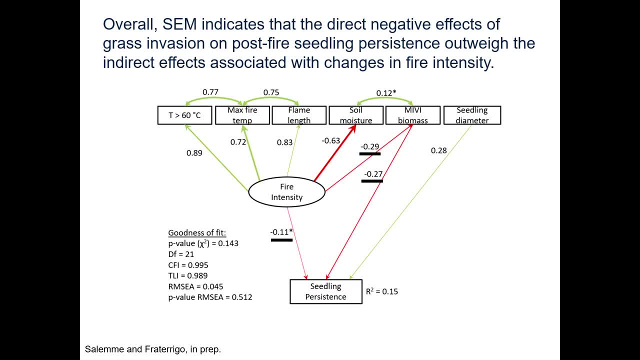 and what I want to draw your attention to is just these underlined values. So these you can think of as the relative support for a given pathway. So fire intensity: as you can see, as we'd expect, there's a negative relationship with soil moisture. 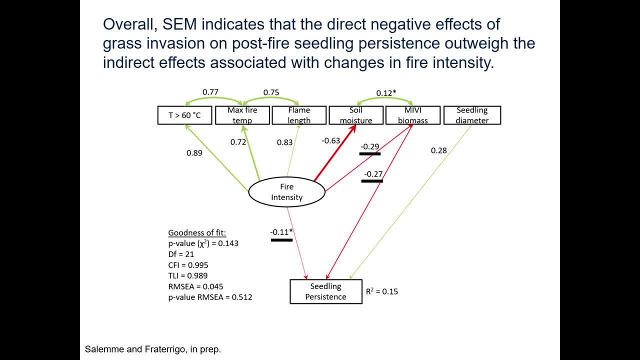 Fire intensity declines as moisture increases. That makes sense. There's a positive relationship between moisture and microstegium biomass. That makes sense. We found in this study a negative relationship between biomass and fire intensity. So as biomass increases, fire intensity declines. 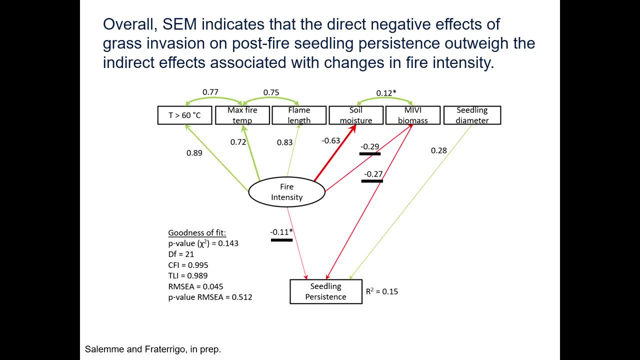 and that's again probably due to this moisture relationship And overall there's a negative effect of fire intensity on seedling persistence. Okay, that makes sense. If it's a hotter fire you should have fewer individuals surviving, But you can see the weight of the evidence. 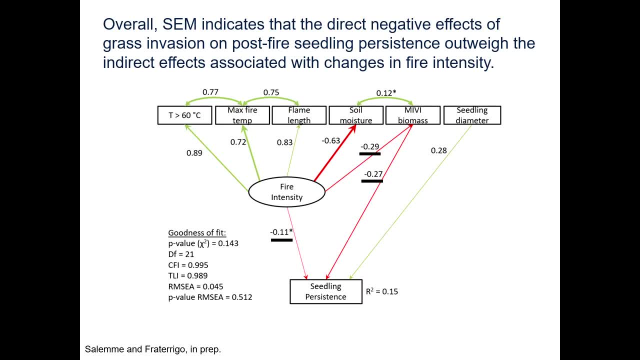 suggests that there's a stronger role for the actual direct effects of microstegium biomass on seedling persistence, Again supporting this idea that it's this direct effect, probably through resource competition, that's leading to less ability of these seedlings to tolerate fire. 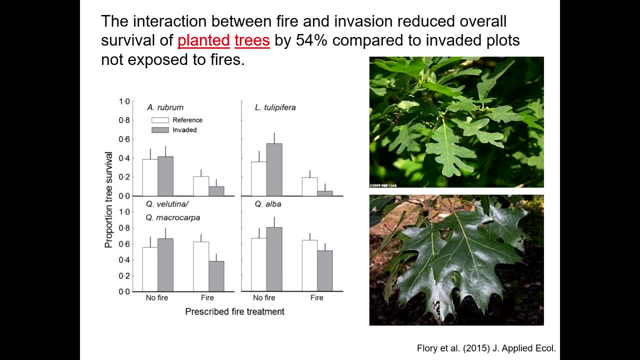 Just to mention, because I think it's important again for this audience to consider, that there's been other work showing that fire and invasion, and particularly invasion by microstegium and verminium, can have these very adverse effects on woody seedlings. 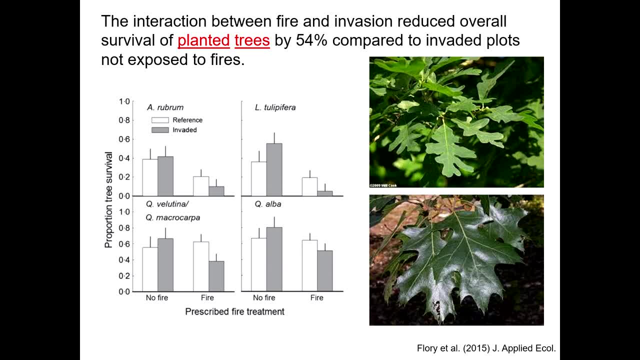 This work was conducted by Luke Flory and others in central Indiana and they showed that fire reduced survival of planted trees. So that's one difference between our study and their study was they were using trees that they had planted. Those trees most likely had fewer reserves. 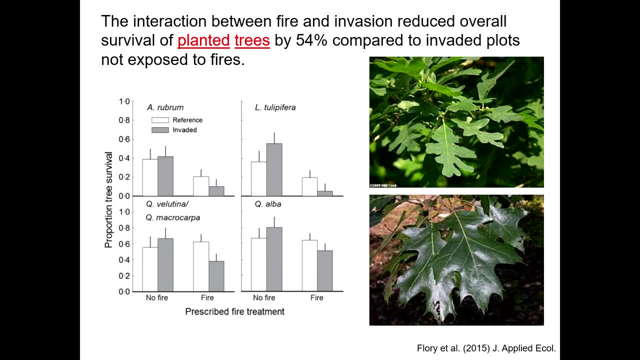 in terms of the amount of carbohydrates stored in their roots and may have been less able to recover from fire as compared to the individuals that naturally recolonized in our study. So that could be one reason that they saw such strong negative effects and the effects that we found. 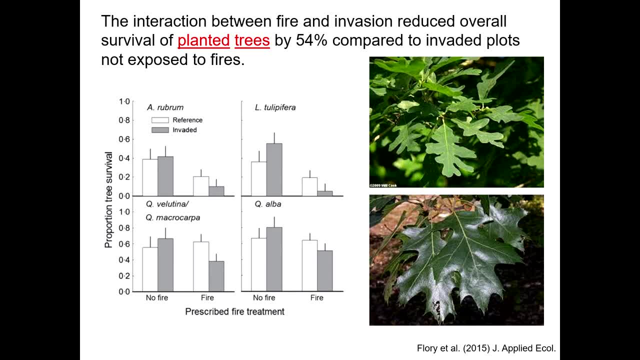 were much weaker. Another difference is they were working in a system where they were burning the fires at sort of the most fire-conducive times of the year, so hot, dry conditions- They saw very intense fires as compared to the system where we worked. 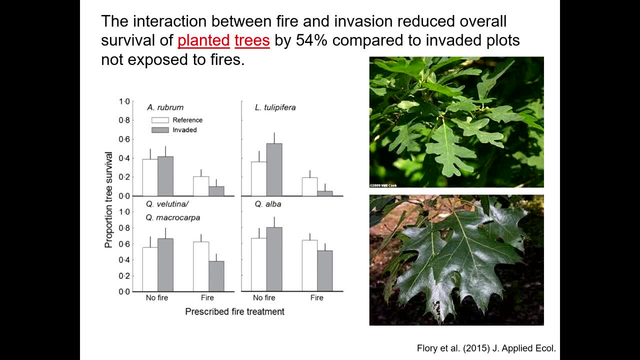 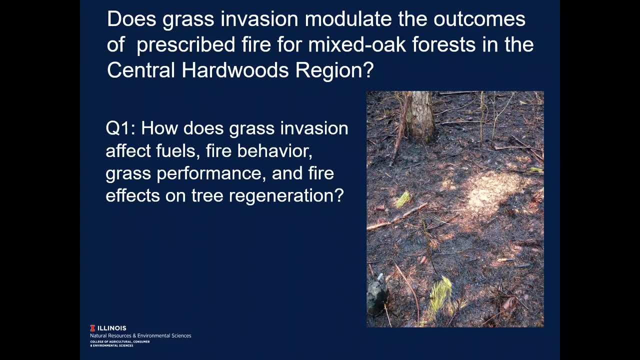 which those burns were mainly happening during the dormant season, which tend to be cooler and wetter. So that's just one thing to keep in mind when considering these two studies together. So I'm going to spend just a little bit of time addressing this question of how does repeated fire? 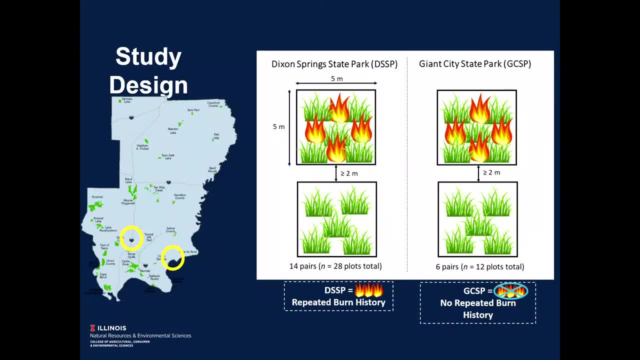 affect the feedback between invasion and fire. So this work is conducted also in southern Illinois, but this time in Dixon Springs State Park and Giant City State Park, and this is work led by Mara Rembelski. So these two sites differed mainly in terms of their burn histories. 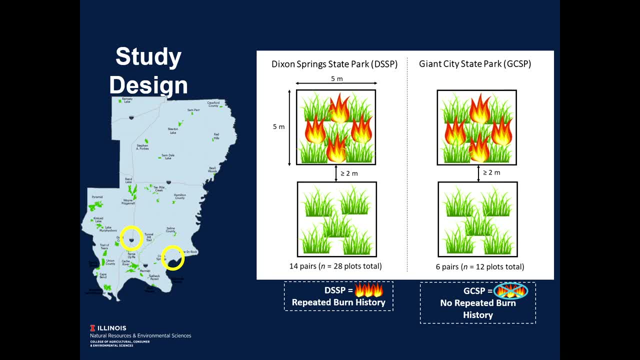 So Dixon Springs State Park has a history of repeated burning. The fire return interval was approximately four to five years over about a 20-year time period, whereas Giant City State Park really had no history of burning at all. So we had a design where we introduced fire. 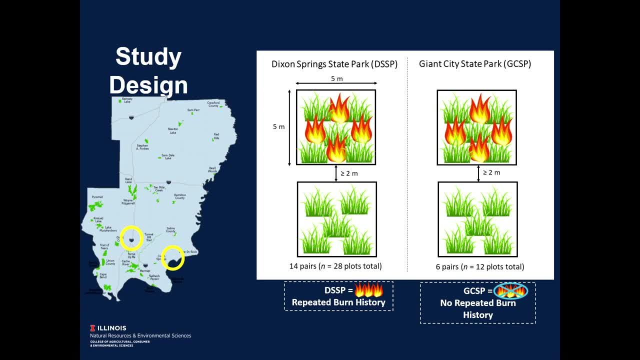 in small plots here paired those with plots that were not burned in that particular year, But again, this is overlaid on top of this fire or burn history. So this allowed us to address this question, though, of, again, the role of fire history. 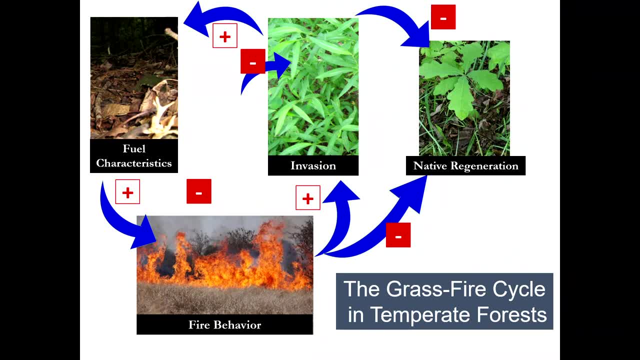 as well as a one-time fire. So I want to come back to this model of the grass-fire cycle and introduce one more player here, and that is nitrogen. So nitrogen is important in this story because we know from previous studies that microstegium tends to like 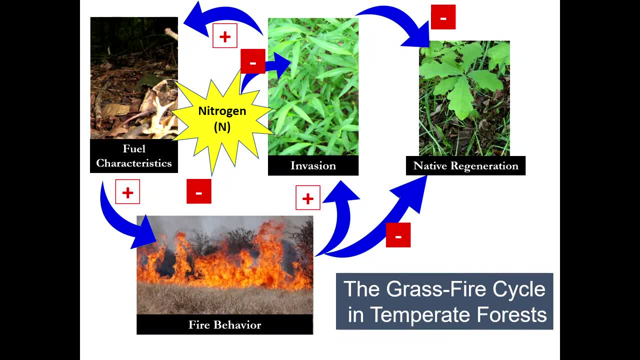 not only moist conditions but high fertility conditions, so places where there is ample nitrogen availability. Now one thing it's important to think about is the role of fire in nitrogen availability. So fire can essentially lead to nitrogen loss from systems. So it kind of has these different effects. 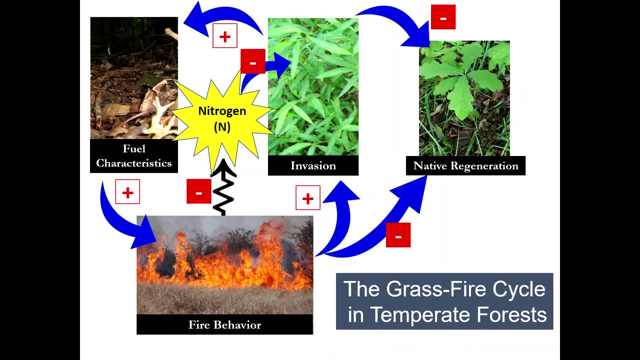 Initially it can convert organic nitrogen to inorganic nitrogen and there's plants or microbes there to take up that inorganic nitrogen. It can stay in the system. So that's often why fire produces this pulse of biomass and growth initially, But in many cases 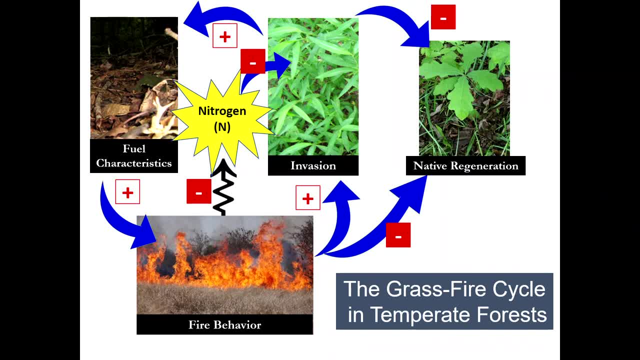 like where we have these dormant season burns. there's nothing to take up that nitrogen once it's converted to inorganic forms, And those forms are very mobile, In other words they can leave the system if there's a big rain event or something else that causes them to be. 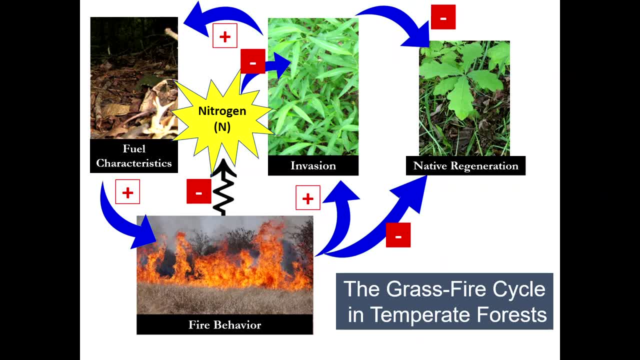 something else that causes the nitrogen to be washed away. So that's one pathway by which nitrogen can be lost. Another pathway is by combustion itself. So if these fires are hot enough, we can actually have volatilization of that nitrogen and it can leave the system in gaseous forms. 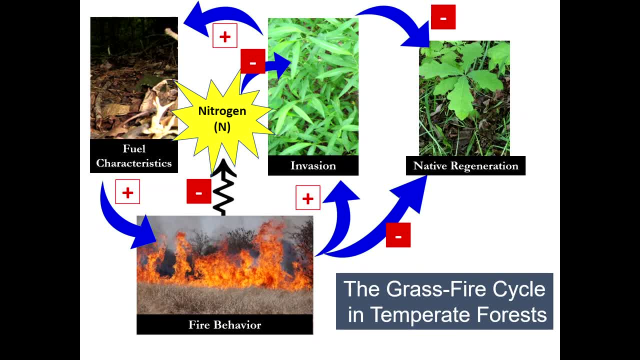 So nitrogen could actually be depleted through fire And again, if we have evidence that invasion is increasing fire intensity, that may lead to greater losses And over time we hypothesize that that could actually have a negative feedback on invasion. Because if these species really prefer areas, 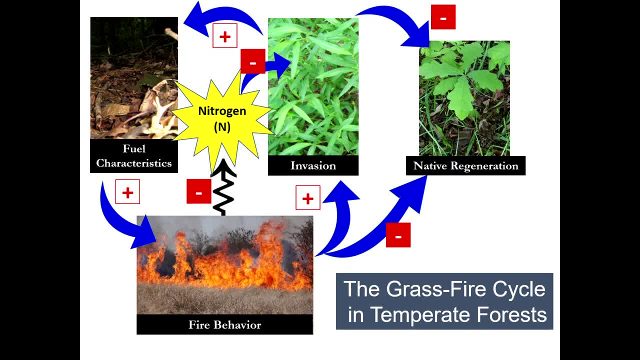 where there's abundant nitrogen available and now we have nitrogen being lost from the system. perhaps over time we actually may see that in terms of the, in terms of a reduction in the severity of the invasion. So we're going to really just talk about 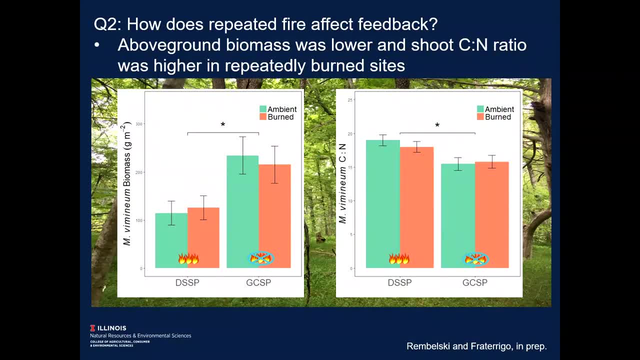 this side of this cycle in the next few slides. So we went out, The royal weaned, The royal weaned went out and sampled these communities that had different burn histories And again I'm just going to focus on the microstegium biomass results. 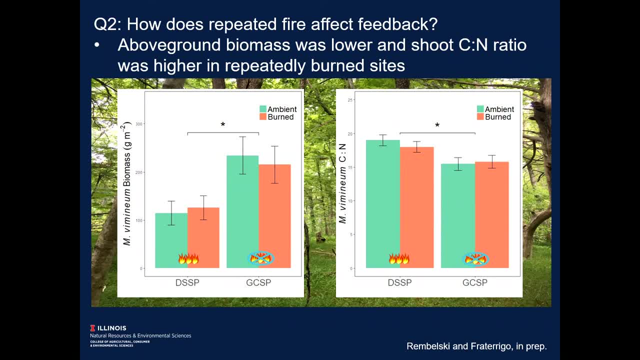 So this is- These are results showing the differences in above-ground biomass. So that is just the shoots part. So we've got again these different things going on. We've got the two different sites: Dixon Springs, where we have the repeated burning. 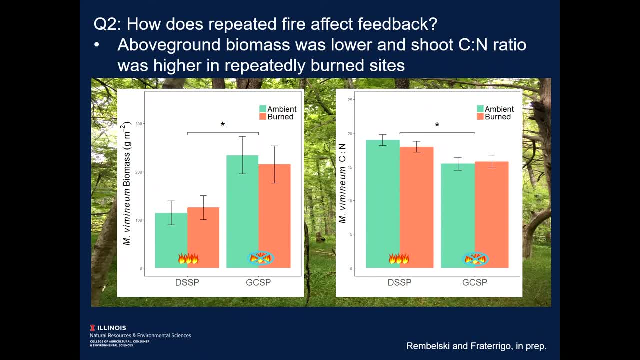 and Giant City, where there's really no history of burning, And then the two different colored bars in each case refer to whether it was sort of our control, ambient conditions- or whether it had there had been a one-time burn in the winter, early spring period. 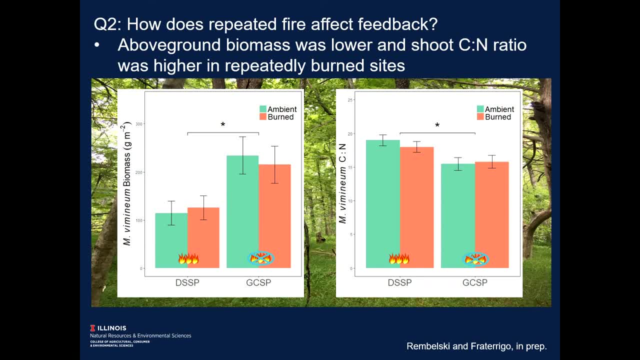 And what we see is, overall, this pretty big difference in terms of above-ground biomass of stiltgrass between Dixon Springs and Giant City. So there's no big difference between the treatments that one-time burn, but big differences between the sites aligning with those differences. 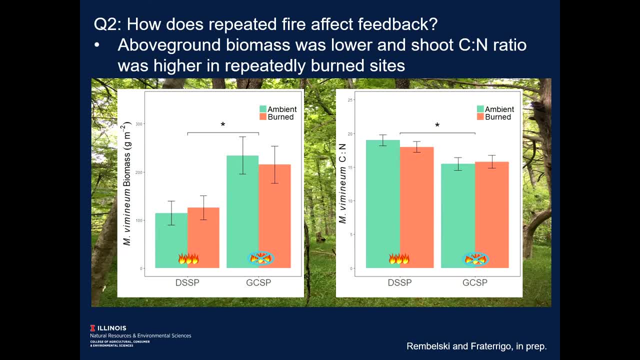 in fire history. So much less biomass in the repeatedly burned sites, And this is the ratio of carbon to nitrogen that we measure in the above-ground biomass, so in the shoot itself, And what we see is a lot more carbon relative to nitrogen in the shoots of the stiltgrass. 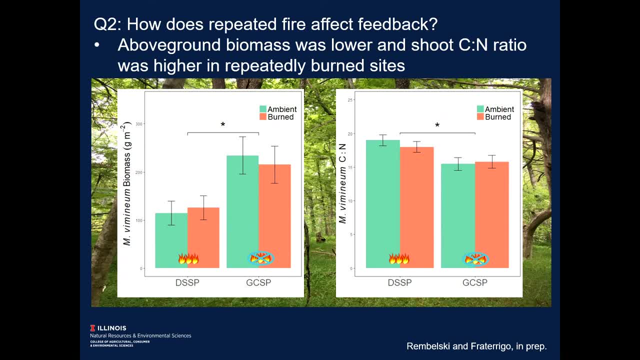 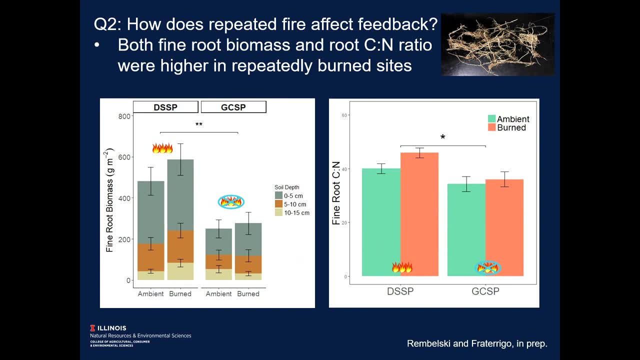 in this repeatedly burned site, as compared to the site with no fire history. Okay, We look below ground too. so that's the shoots. What about the roots? The roots show a consistent pattern in terms of potentially supporting the story of nitrogen limitation. 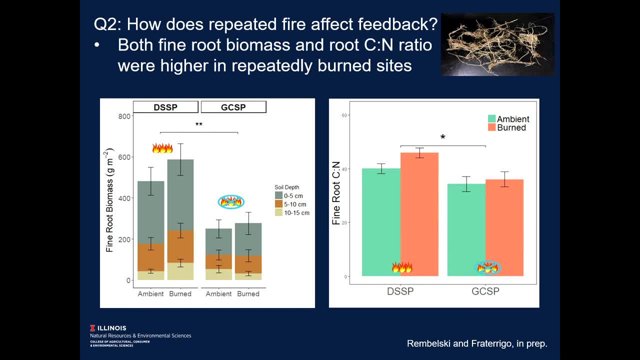 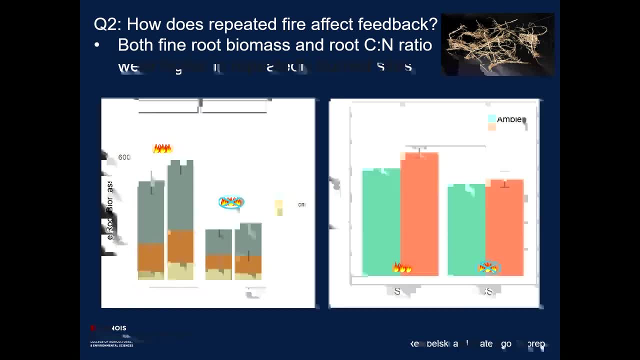 So fine roots. you can see there's much greater carbon investment. so just the amount of fine root biomass is much greater in the Dixon Springs study site, which is the site, again, that had been repeatedly burned over 20 years. So in other words, plants are investing. 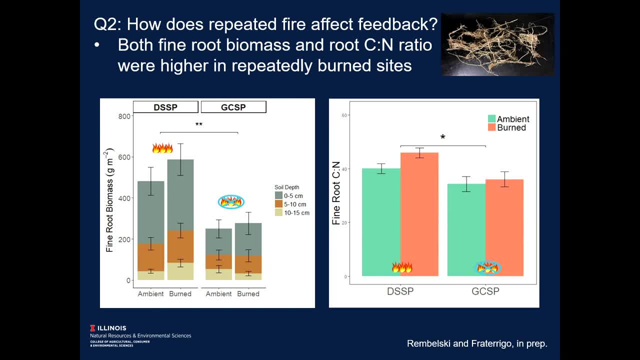 a lot of energy and carbon in producing roots, And one reason they may do that again is because if nitrogen is limiting, they're going to need to explore more volume of soil in order to take up more nitrogen to support their growth. So these shifts in sort of plant allocation of carbon. 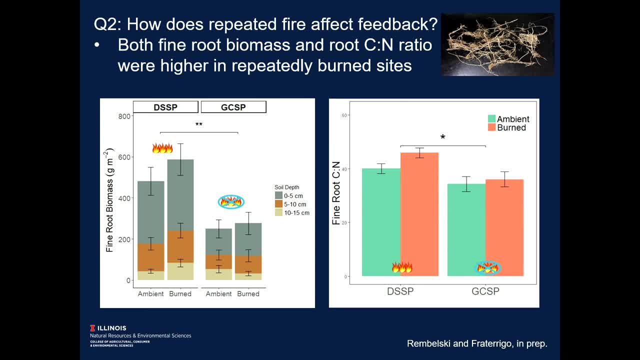 are in line with this notion that nitrogen could be more limiting or is more limiting at Dixon Springs as compared to Giant City. The carbon to nitrogen ratio of the fine roots also supports that, so we see more carbon relative to nitrogen again in Dixon Springs. 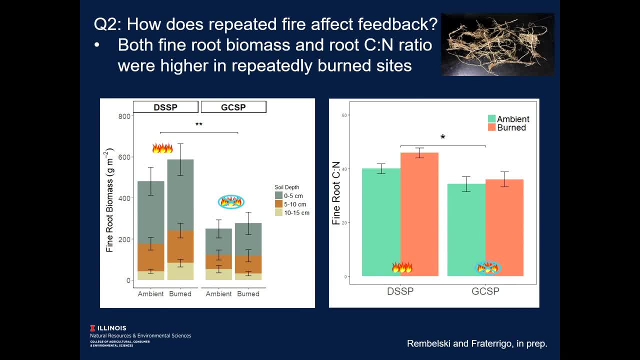 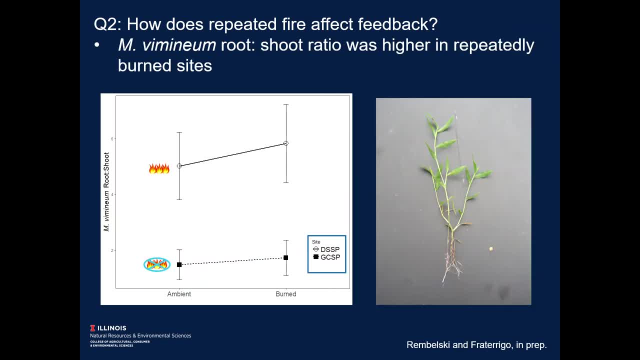 relative to Giant City. So, overall, suggesting less nitrogen being available here as compared to Giant City. And if we look at the two, the biomass in the shoots compared to the biomass in the roots or, I'm sorry, the other way around. 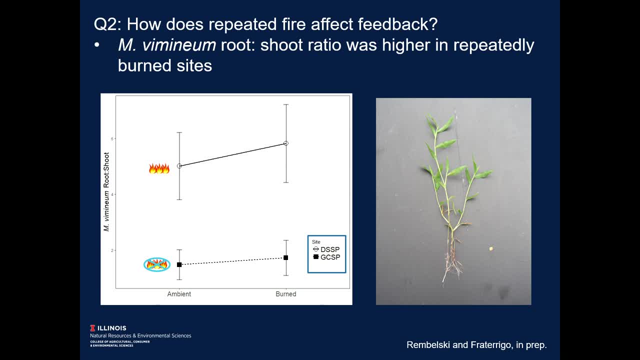 biomass in the roots compared to the shoots. similar patterns emerge in the repeatedly burned sites have, overall, much higher biomass in the roots as compared to the shoots. Okay, so just the difference in these lines, and we see very weak effects of that one-time burn on this pattern. 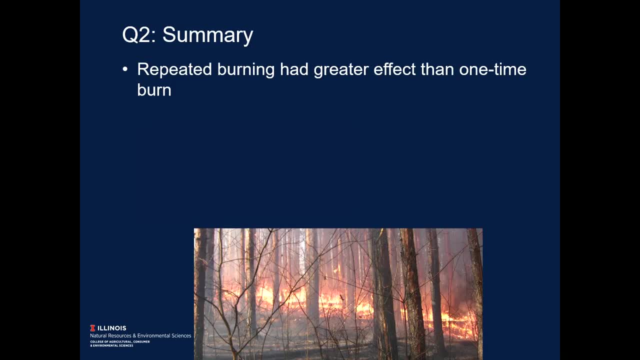 Okay to summarize those results. then repeated burning led to a greater effect than one-time burning and also we see evidence of a larger investment in the roots versus the shoots, consistent with nitrogen limitation. Shoot and root C to N ratios also support that line. 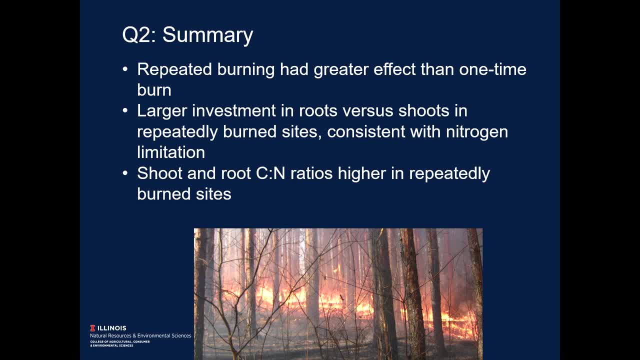 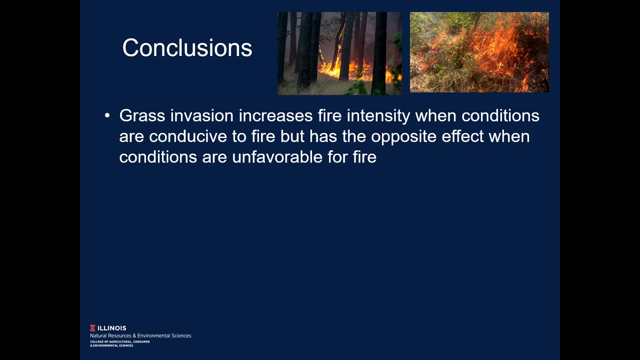 in terms of there being higher C to N ratios in the repeatedly burned sites. So, just to conclude, across all these studies we've seen that grass invasion- there is evidence that it can increase fire intensity when conditions are conducive to fire. So, again mainly from these studies, 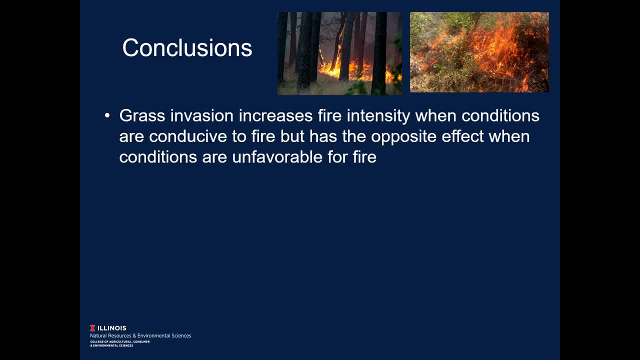 that have been done in Indiana, whereas our work, which follows more of the burn regime being used by the Forest Service and other land managers, really doesn't show that strong of an effect of microstegium on fire intensity, largely because those fires are happening. 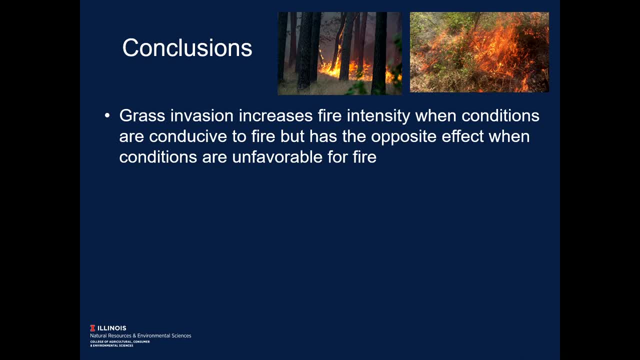 at a time of year which are less conducive to very hot fires. Also, it seems to be the case, based on our evidence, that the direct negative effects are much stronger and outweigh those of the effects of fire intensity on persistence of woody seedlings. 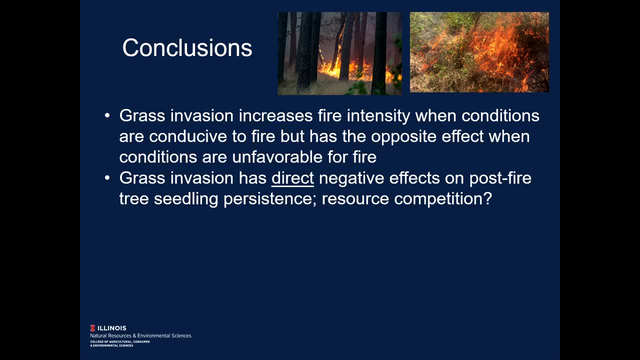 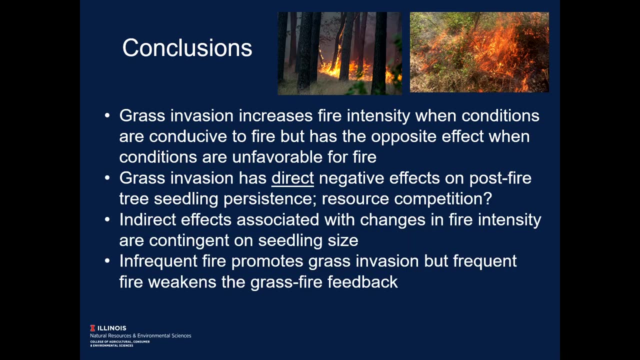 So grass invasions have this direct negative effect on post-fire persistence and this, like I said, could be very much related to resource competition, As I pointed out. those indirect effects were present, but smaller and contingent on seedling size. And then, finally, 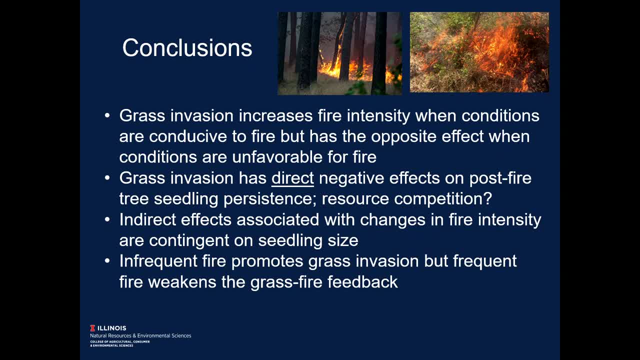 our evidence suggests that infrequent fire, while it promotes grass invasion, repeated burning is actually weakening this grass fire feedback. I do want to just mention the caveat that these species persist in the understory. They're just not as vigorous invasions after repeated burning. 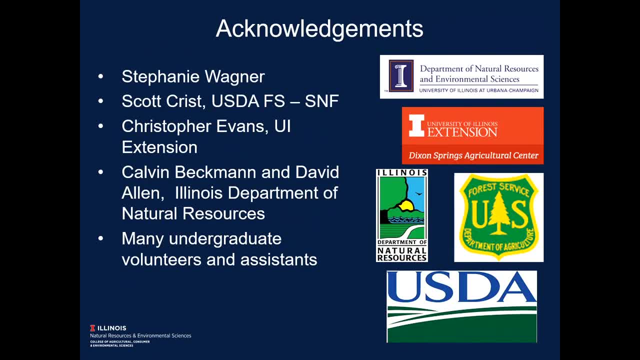 but they're still present. Okay, And just to acknowledge people who've assisted with this work and support from different funding agencies, and I don't know how I am on time, if there's time or not for questions. We've got a couple. 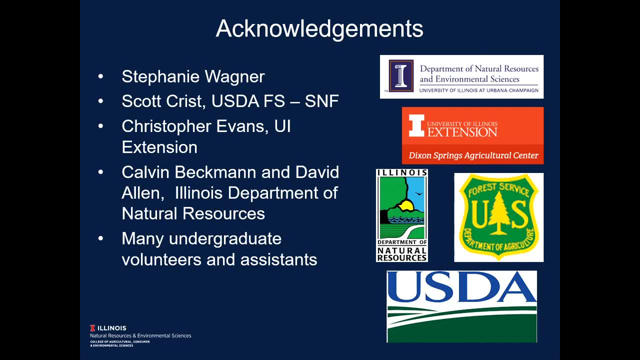 Couple minutes, Okay, So if there are questions, feel free. I've got one. Yeah, You talked about your fire and that impacts the tree seedling persistence? Yes, Did you see a difference on functional groups of seedlings Species? 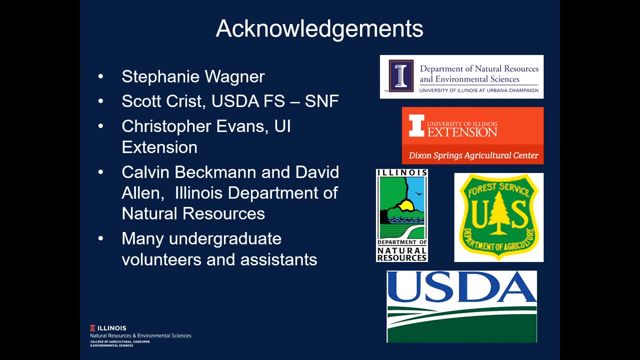 Right, We looked for species effects. We really didn't see strong evidence. You know, specifically we expected that there would be larger effects on your fire intolerance species, but it seems to be really overwritten by that size threshold. So you know, 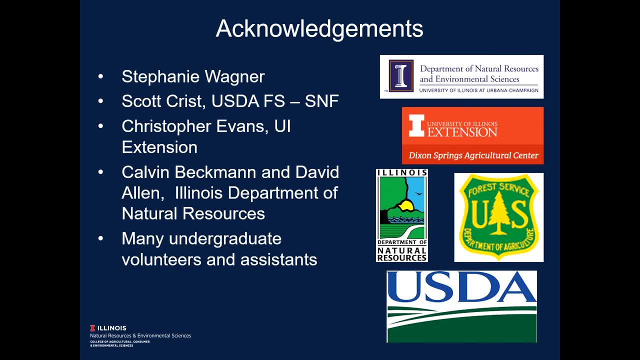 there just wasn't much variation. Now I know that in the flurry study they saw some bigger differences between species. We just didn't see much of that. Yeah, Just How do you measure maximum fire intensity? So you know. 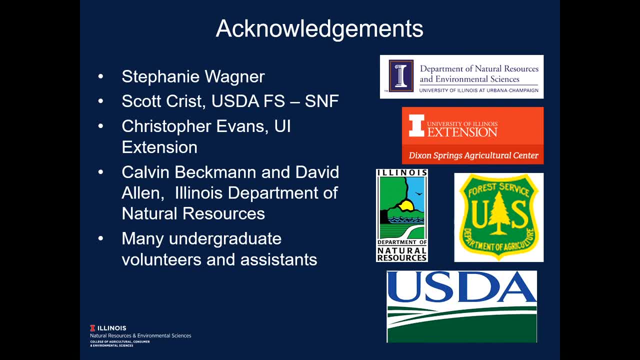 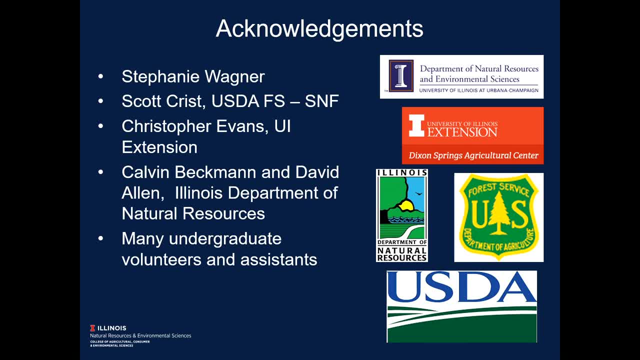 So we had them in, you know, located in different parts of the burn unit that was going to be burned, And they were at right above ground level, Yeah, So capturing kind of surface fire intensity, Yeah, That's a good question. 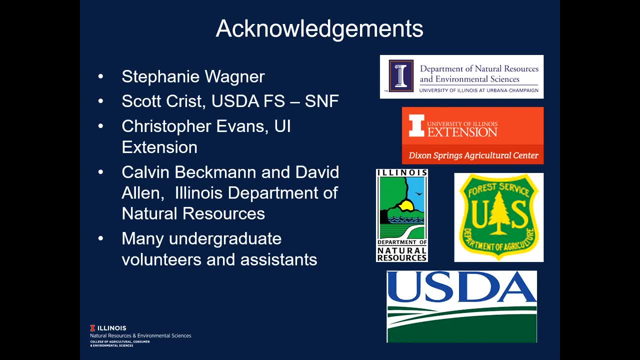 And we also- I didn't present these results, but did other things like use the sort of flame height indicators and things like that. Yeah, So you know, that's a good question And we also- I didn't present these results-